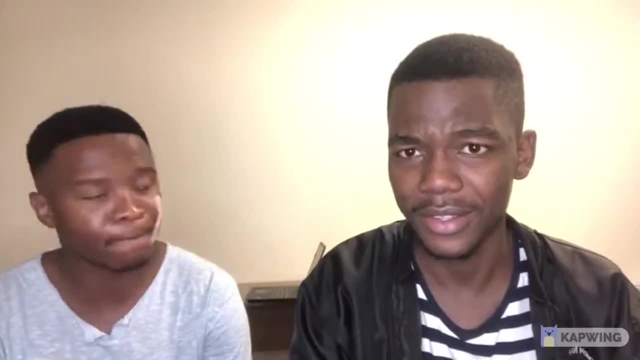 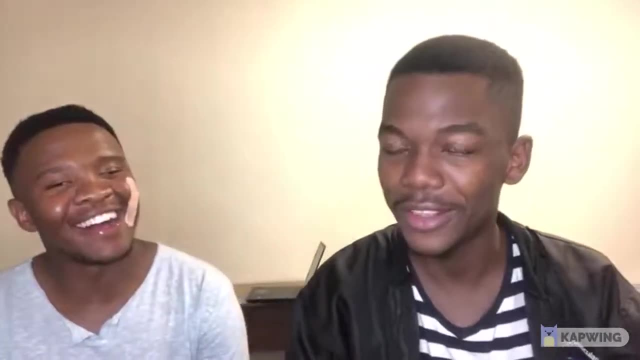 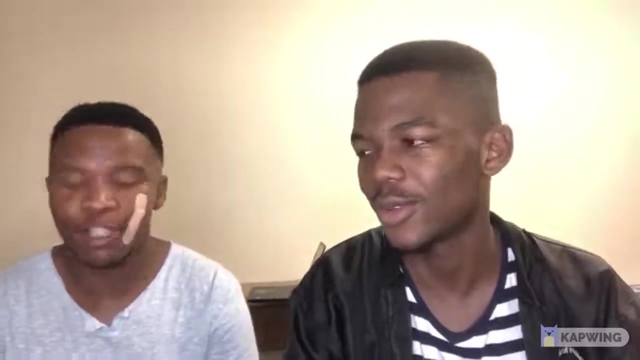 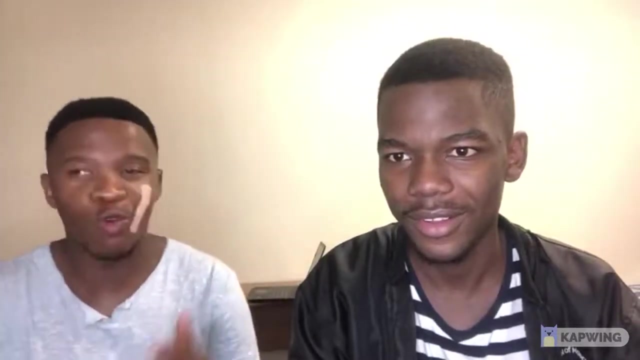 in Fraglacta, number one from Pumzile Secondary School. My man, can you repeat, like slowly, Okay, Doing what We call it Mathematical Statistics, Mathematical Statistics, okay, So that's why in all it's called bachelor in Mathematical Science, with Mathematics and 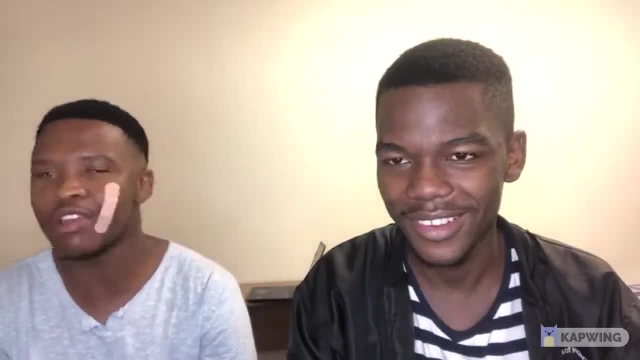 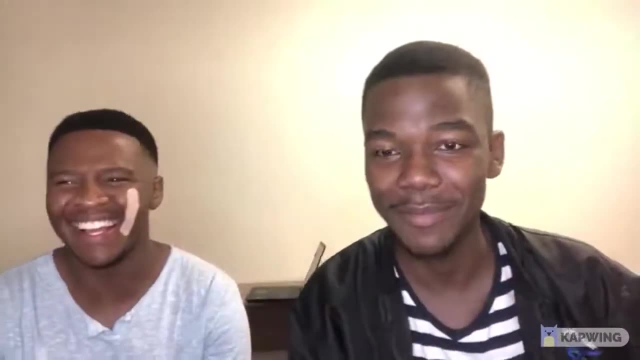 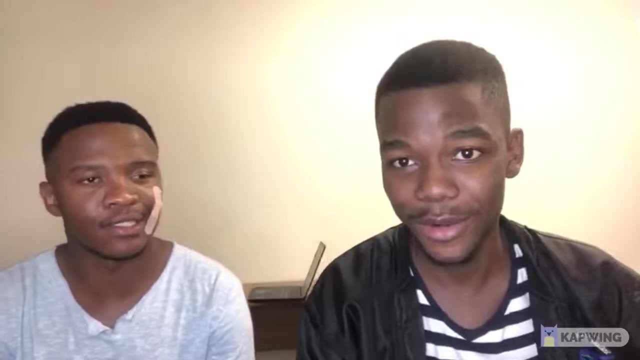 Mathematical Statistics with Financial Orientation. not everyone knows it. Hey, Yeah, Mathematic statistics, mathematical statistics with finance At the end. financial orientation, Financial orientation. Yeah, So let's say, let's just say mathematical statistics, Yes, Yes So. 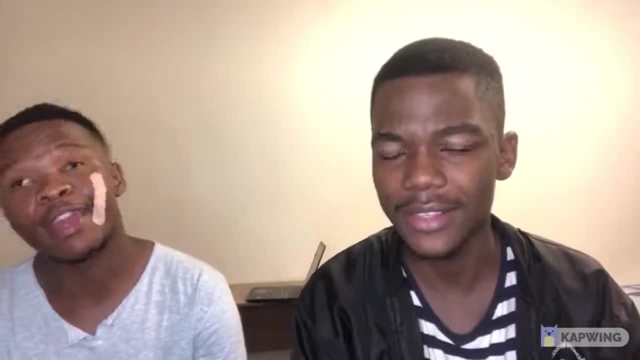 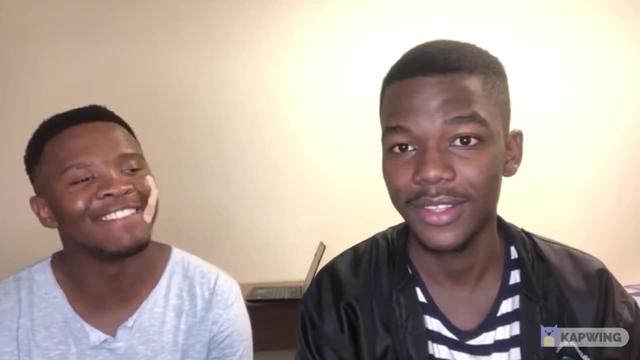 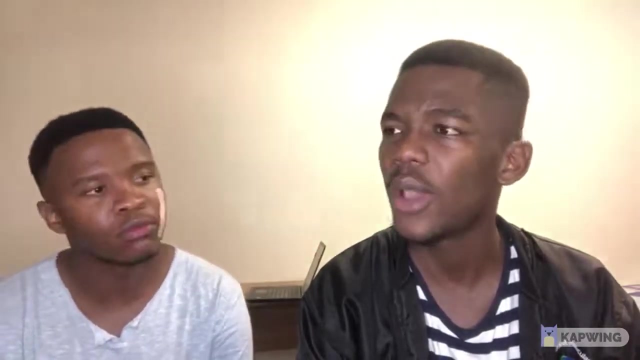 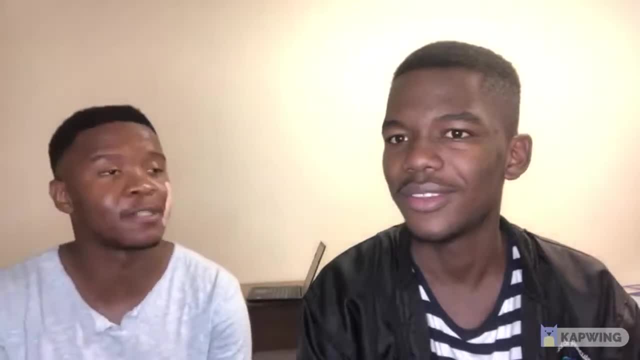 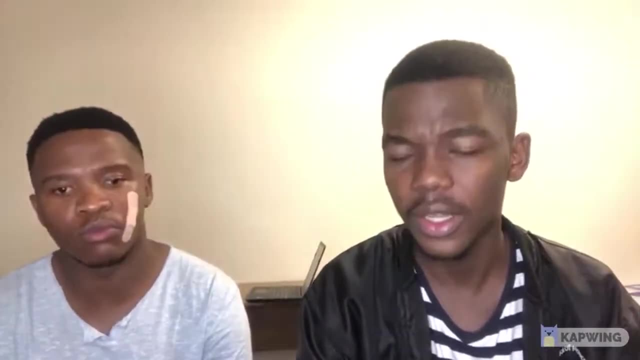 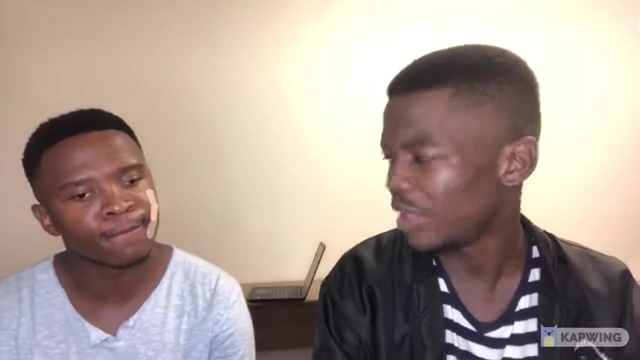 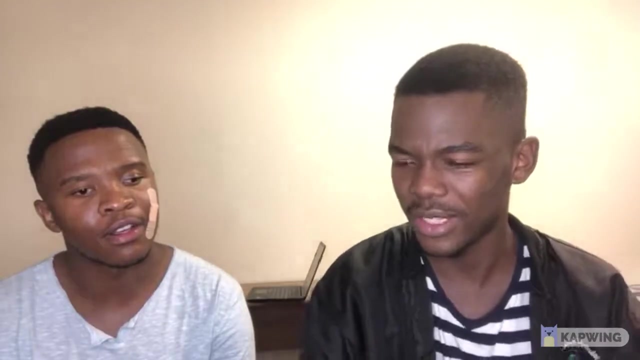 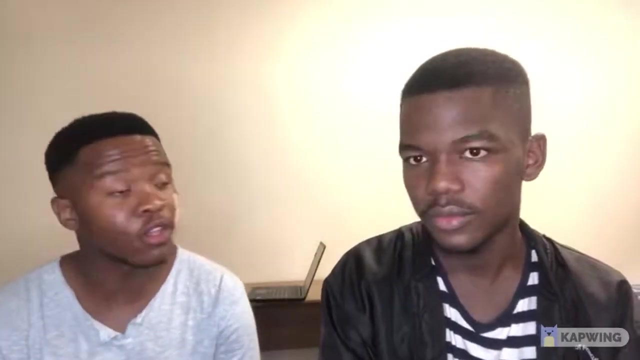 all right, so your high school name. so did you plan to, to, to to study a mathematical statistics? um, in high school, you knew, or there, is there something that you wanted to do, but before you find yourself doing mathematical statistics, oh, the thing is, uh, i knew that i wanted to do something that involves mathematics, but i didn't know that. 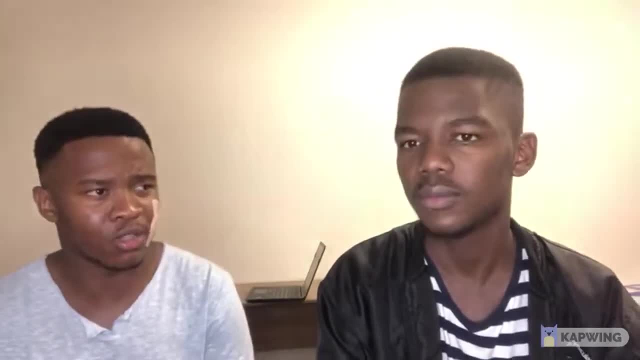 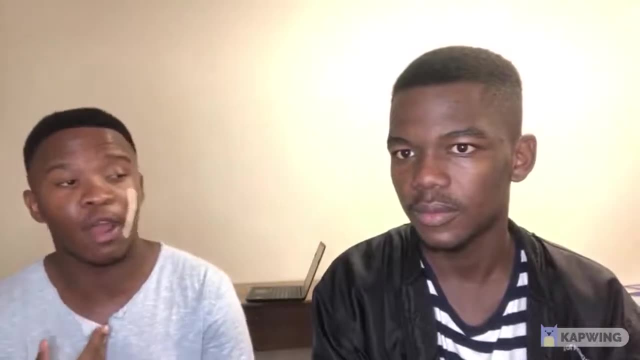 uh, these statistics, there's uh something, something like this, ever so the thing that i wanted is only maths, a course that deals with maths. but when i get to, uh, okay, i wasn't, i didn't apply for myself. so my teacher, mr c toilet doing physics, um, he applied for me, so he chose mathematical statistics. 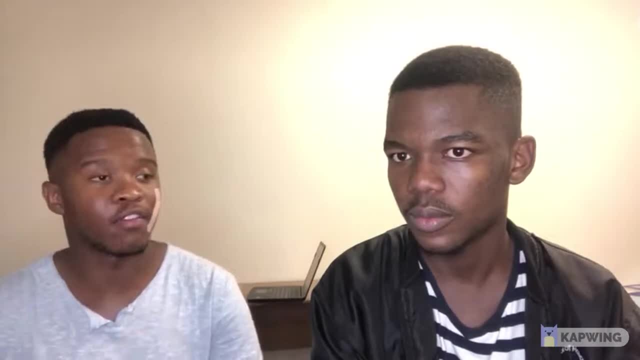 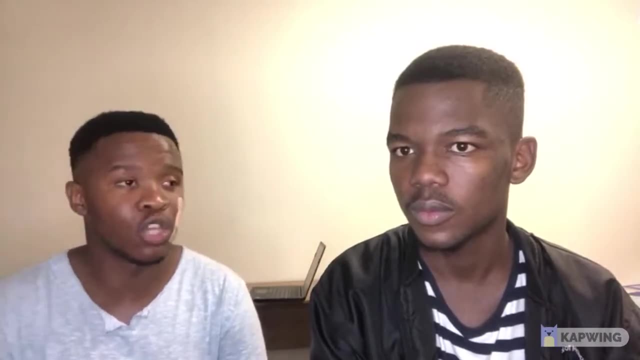 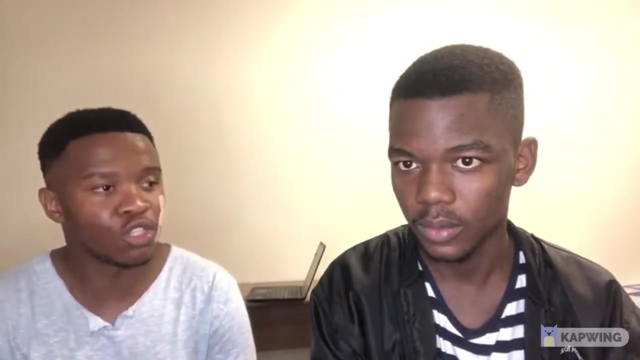 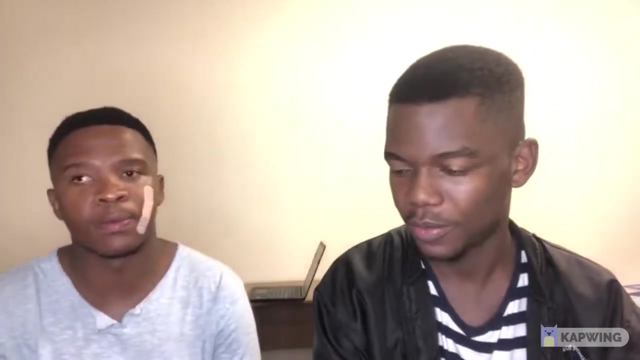 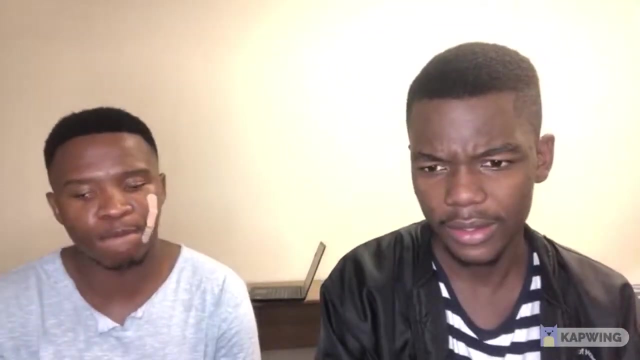 and then i only applied in ug. i didn't apply in other universities. you know, uh, us from back home, we, we are not familiar with this application. he's not a bad cie. yeah, so it was 2020.. yes, first year, all right. so you applied to university of johannesburg? yeah, yeah, well. 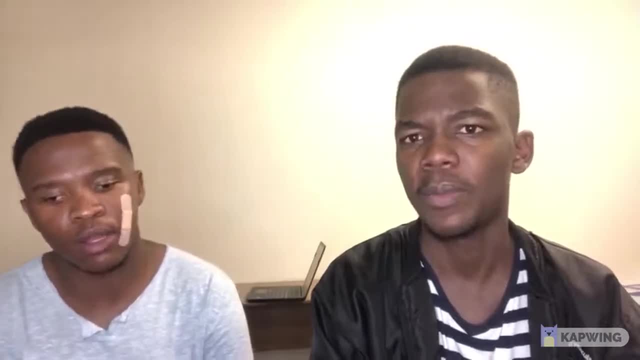 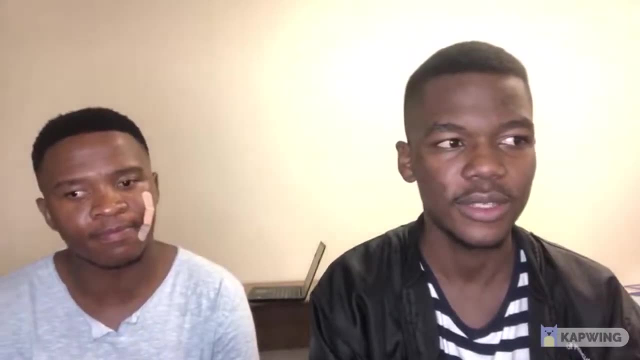 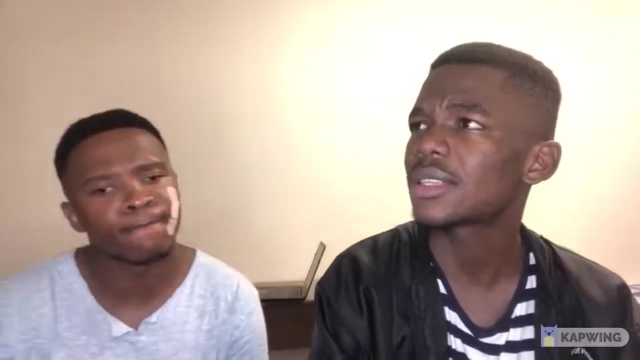 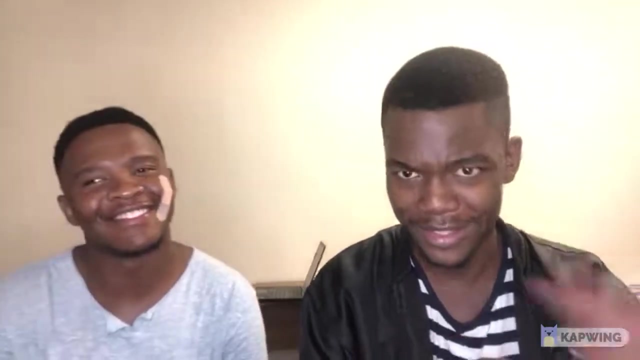 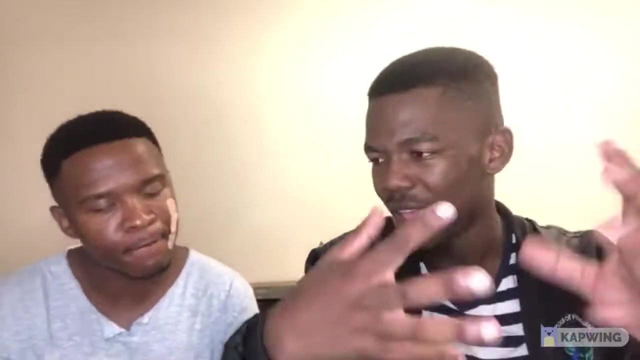 applied to university of johannesburg, yeah, yeah. so university of johannesburg did accept you, yes, started with a mathematical statistic. so uh, tell us now, you, you can see that, uh, mathematics in high school is not the same with mathematics here in university. true, true, true, yeah. so now you, you become a, a mathematical science. 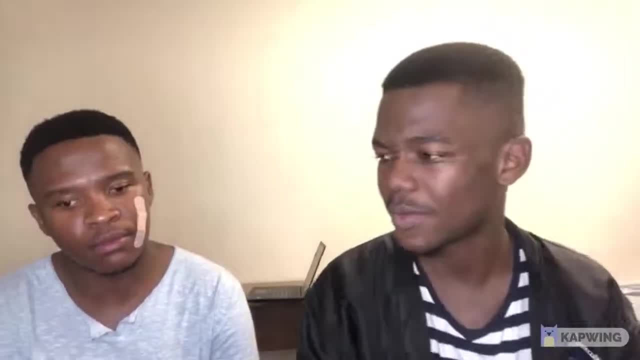 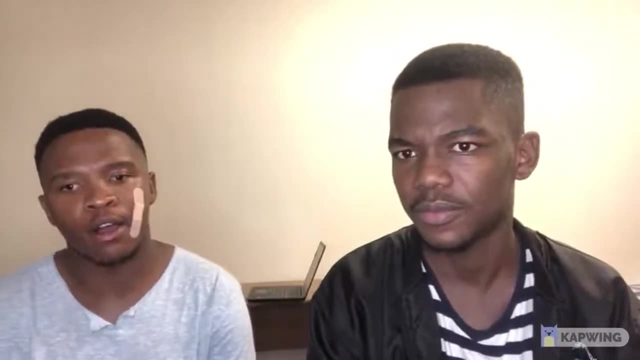 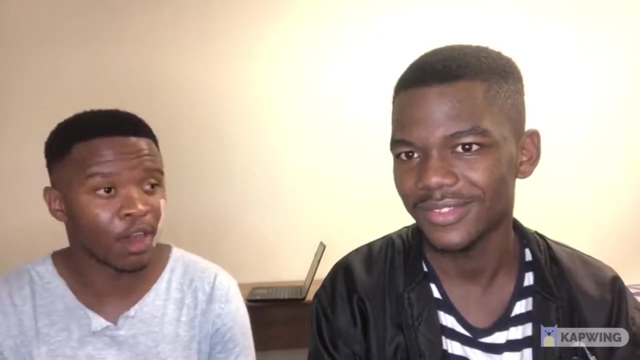 and student, yeah, so tell us. the challenge is now: which modules gave gave you some problem? you get it okay, okay. yeah, um, okay at first. when i got to varsity at last year, 2020, okay, uh, it's not the same as you said. uh, comparing to uh high school, you know, i had in high school you could, um, just 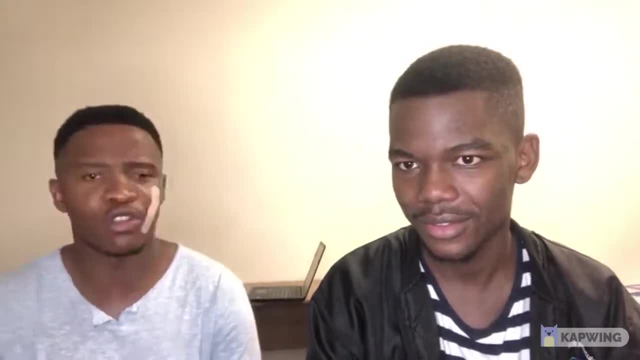 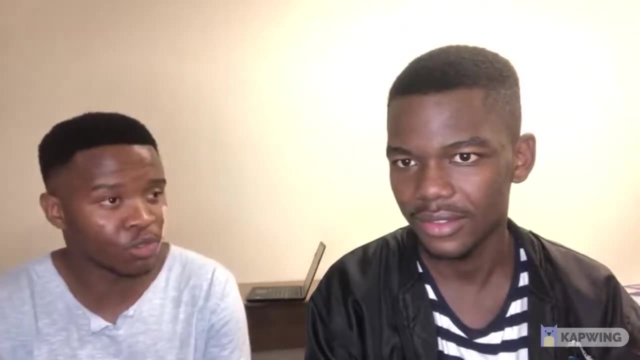 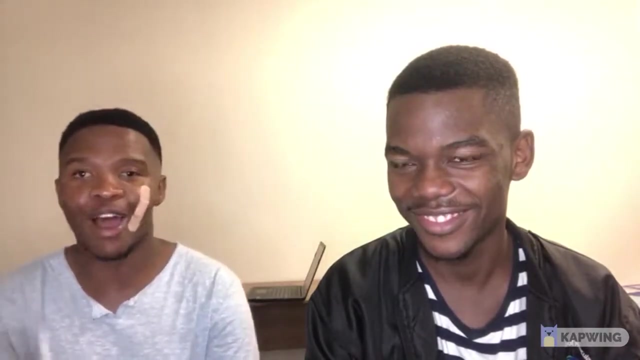 be in class, i understand, and not even study at home, because if you maybe you love meds, you can just hear everything in class, then uh be able to apply uh wherever they need to test you. so when it comes to varsity, okay, my first test, i remember i got less than 50 percent. i was so ahead because 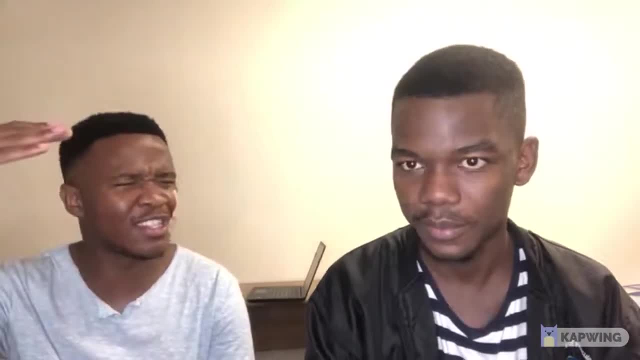 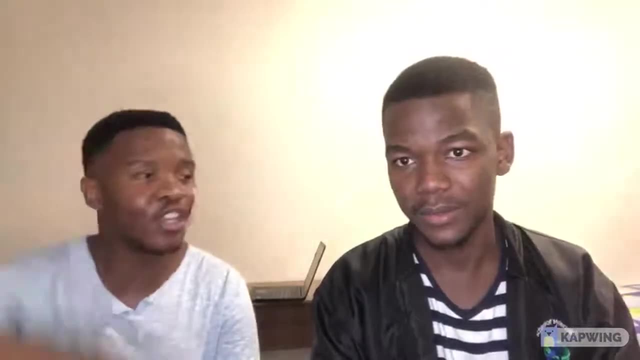 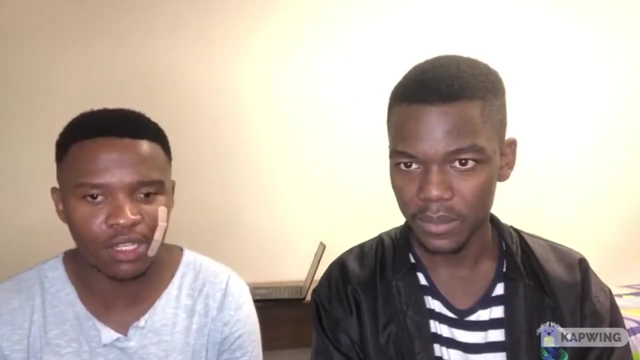 i was uh used to, uh, you know, getting 70s, uh 80s when you get to varsity. that's where you learn: hurry, there is no genius. yeah, we are all equal genders. everyone is only good, you understand. so, okay, um, the challenges that i had uh last. 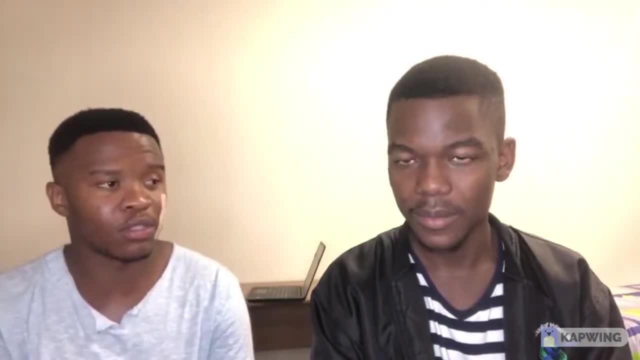 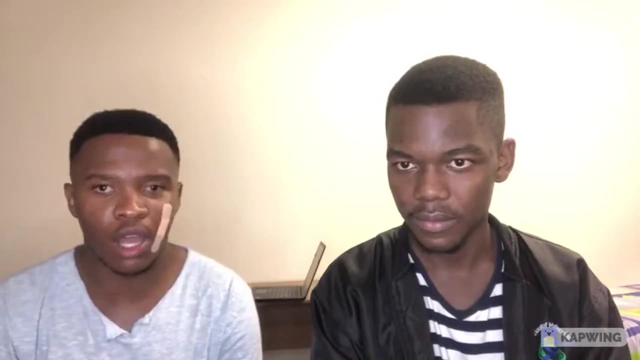 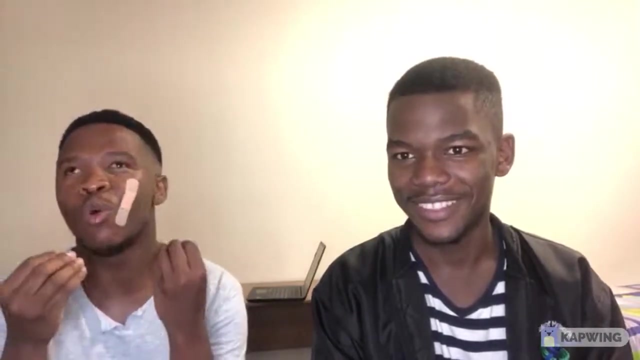 year. mostly is to adapt in a new environment. yeah, like it took me some time to just adapt. you know, make new people, um, and all that, and the modules that i found difficult in, i did, i, i did computer science last year. okay, at some point i didn't know why i was doing it, but it was there, i had to pass. 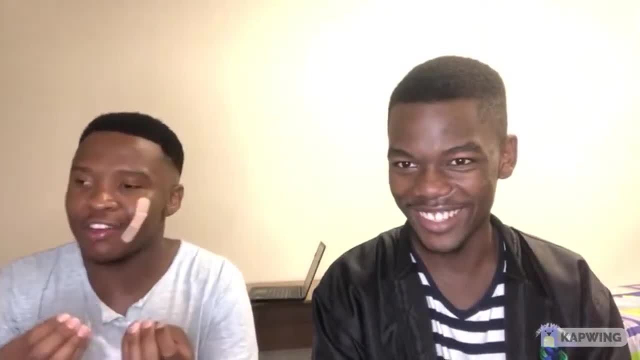 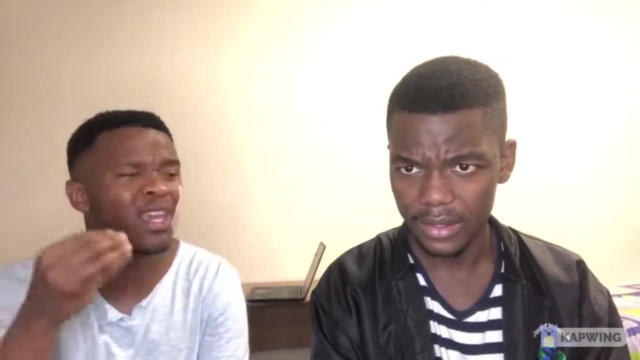 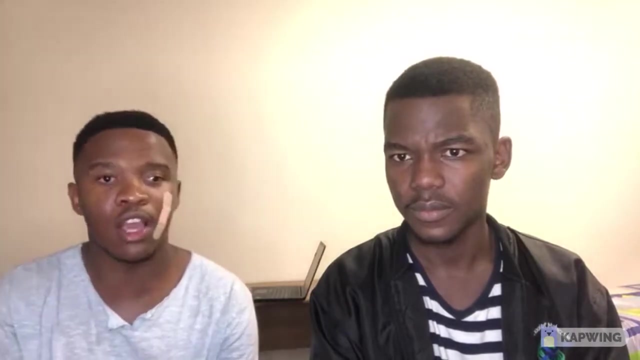 it. yeah, i had to pass it. then, from there, you know the coding, because i remember last year, um june, at the exam i had to be, i was, i was programming a game, you know, and i think it was so difficult, um, you know, at high school. what i noticed is that at high school, uh, it's, there's, there's a lot of work and it's. 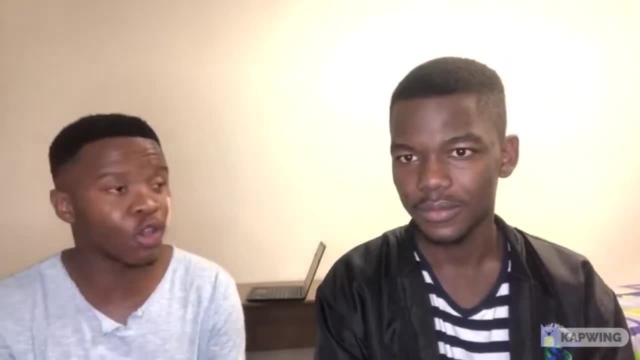 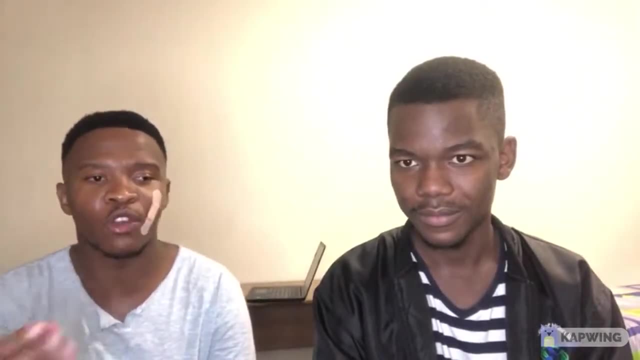 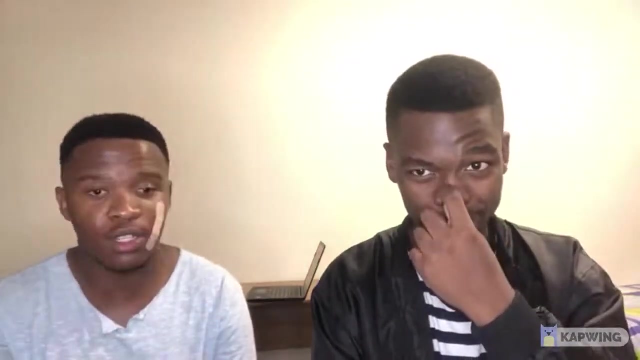 understandable. then here at varsity there is also a lot of work, but it will take you time to understand the content you understand. so it's kind of difficult for us to to just grab everything like we did in high school. so the challenge is we're just adopting a new environment and some modules are like computer science and in maths. 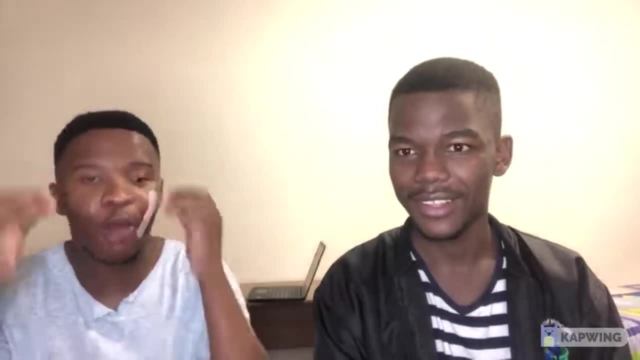 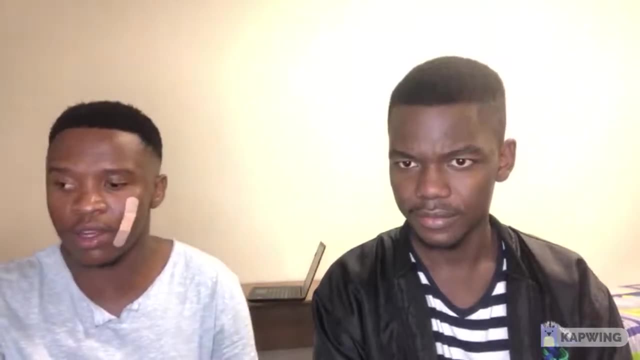 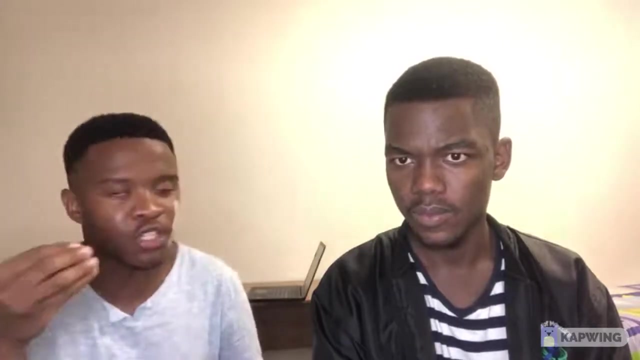 the formulas are changing. you know and you have to know them by heart. okay, instead you have to know them like if, if, uh, they give you, uh, something that you have to, um, uh, let's say, evaluate at first, you have to look at it, analyze it and know which formula you're going to apply. just have an idea. 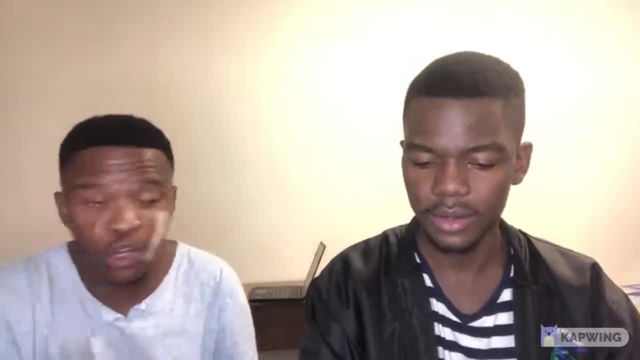 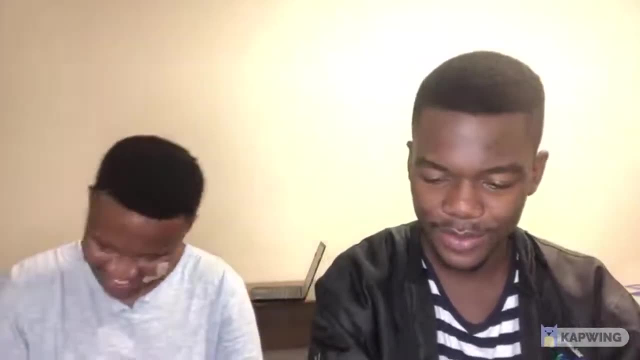 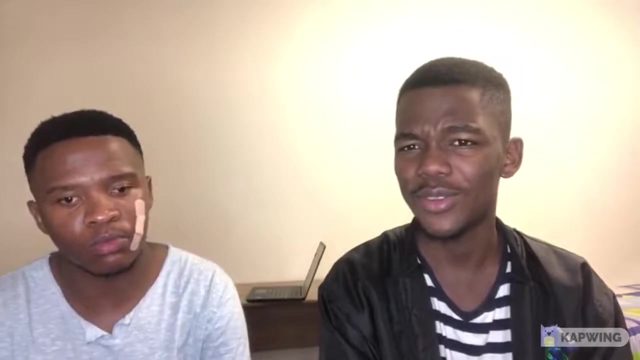 on what you're going to do. that's meant because if you don't know what you're going to do, you won't. wow, yeah, computer science, mathematics, yeah. so how did you cope with, how did you manage to pass this computer science, computer science, because i'm sure there's someone who's taking statistics. 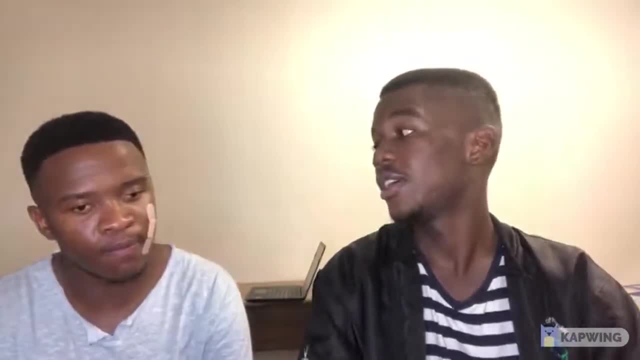 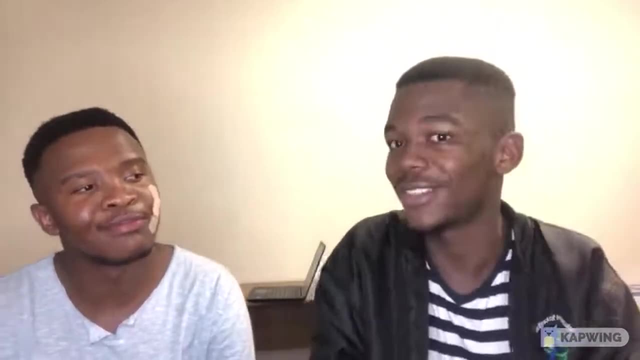 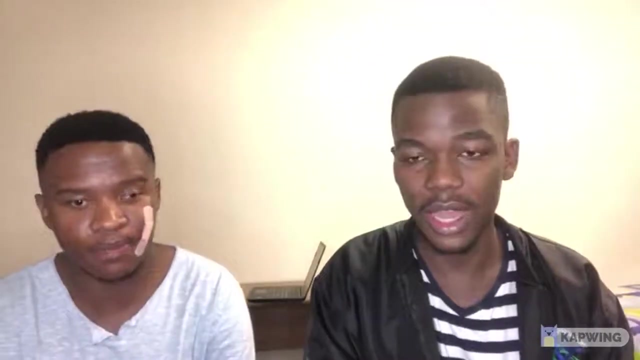 watching us. yeah, yeah, he or she will find it him or herself doing that computer science module. even though maybe it's not that, maybe it's important. they know why they put it in there. yeah, yeah, yeah, because they are it is. you need that coding ability, that's true. so how did you manage? 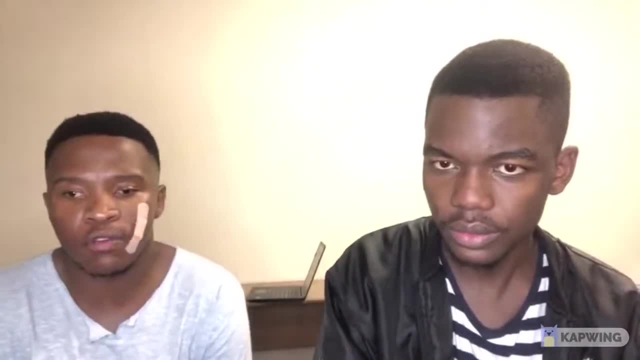 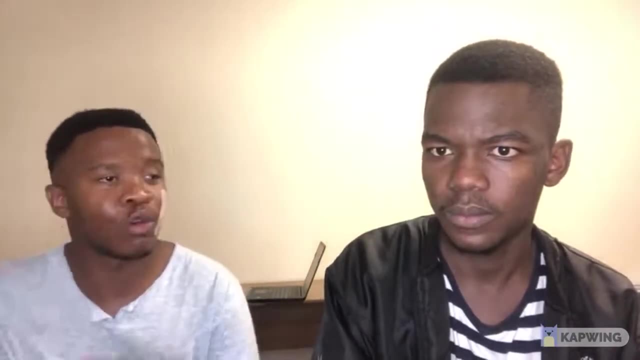 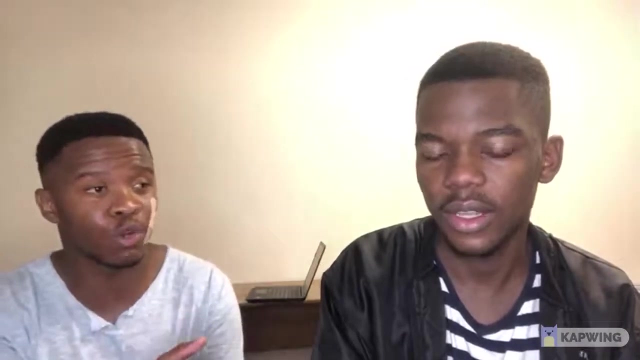 um, you know what, what i thought of doing last year? uh, firstly, i started to have friends. you know, i had friends um from all over. you know, i didn't um like exclude myself from everything i wanted to be in, you know, but only on academic issues, not like uh exclusive things, no academic. so uh there, 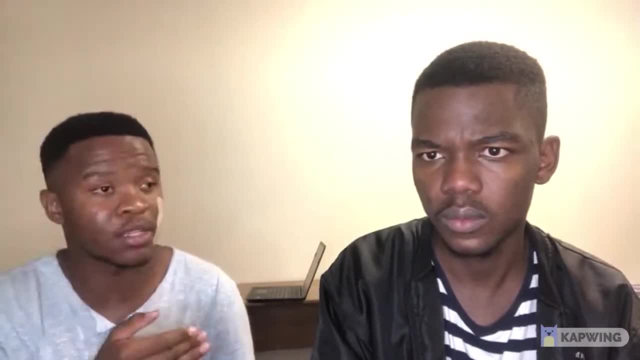 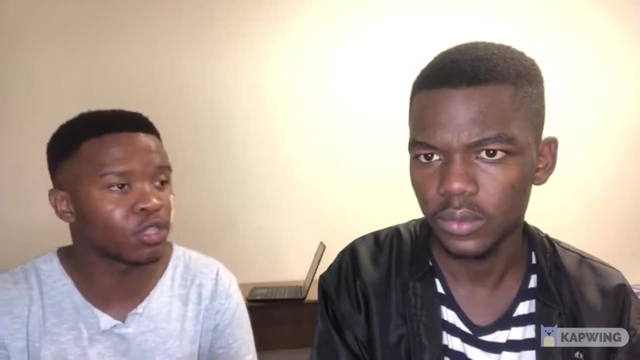 you know, uh, everything is there. remember, after mathematical stars we were meeting uh at the d labs. you know, then from there we will uh just combine everything that you know about computer science. then we'll just combine everything, then we're gonna uh make something happen, you know. 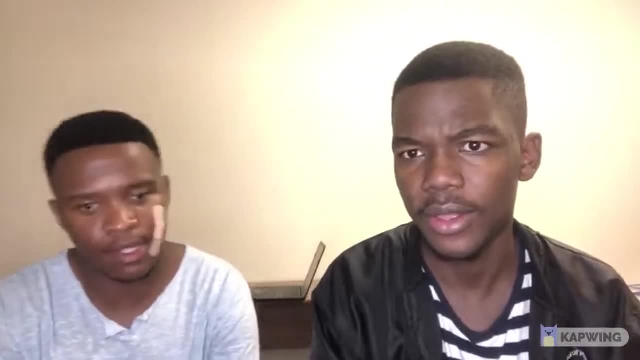 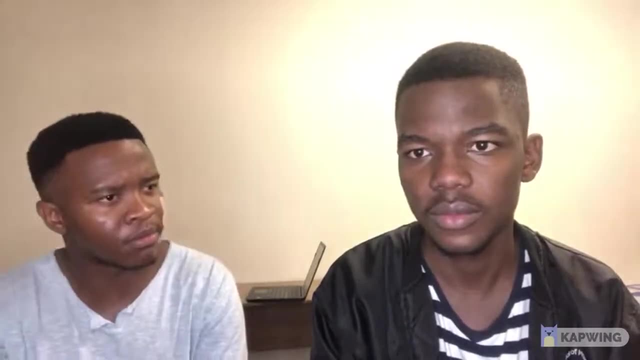 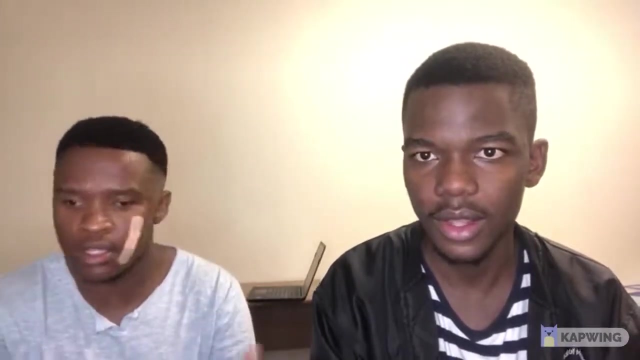 not just only a study partner, a study group. yes, yes, like have people? not right now. there are many people who i work with through whatsapp. i never met them, but you are working. like how can we set up a meeting in uh bbs with this uh content that's in that thing. 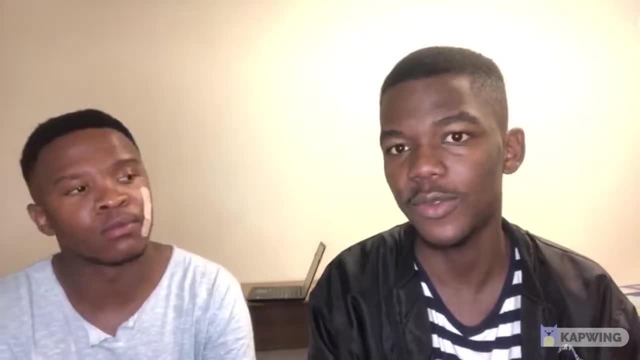 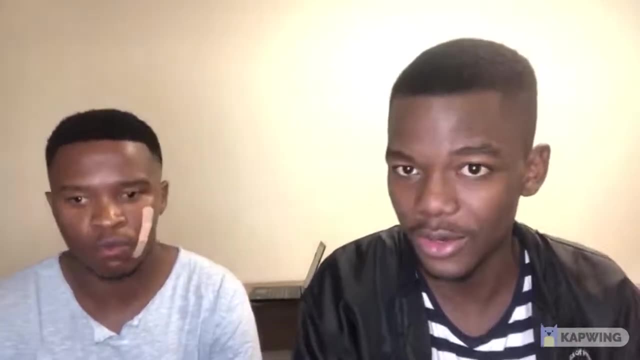 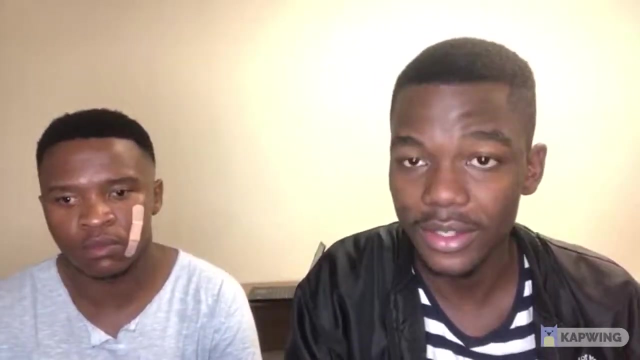 that was a great advice. yeah, because i'm sure even if you have, if you are six guys like about maybe the majority of the people, maybe they will understand what you're doing- they can be able to to help you, that's true. so in all, it means that when you finally reach university, you must try and 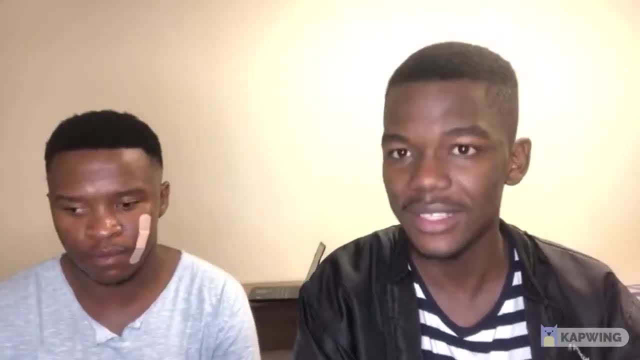 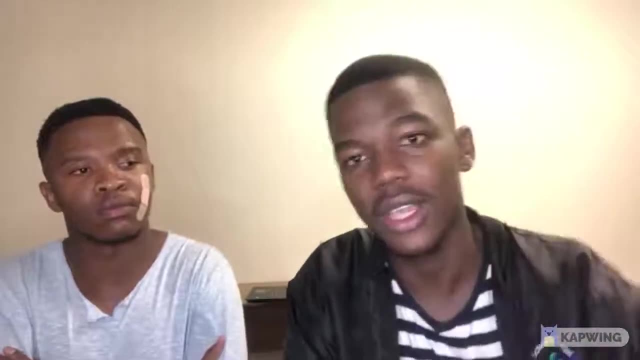 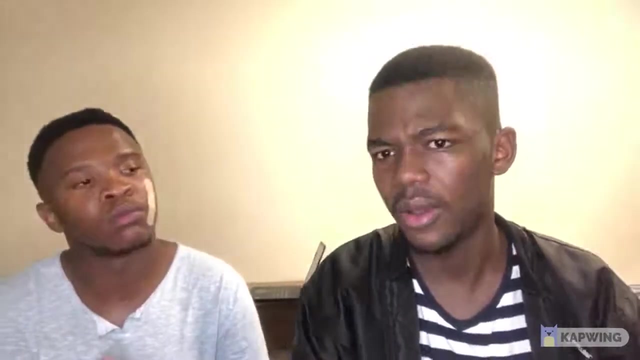 find a study group, a study group that you trust, in order for you to be able to, I would say, some of the students in those groups. they could help you understand the content much better. Yeah, that's true. So now, if I have a degree in mathematical statistics, I can work as a watch. 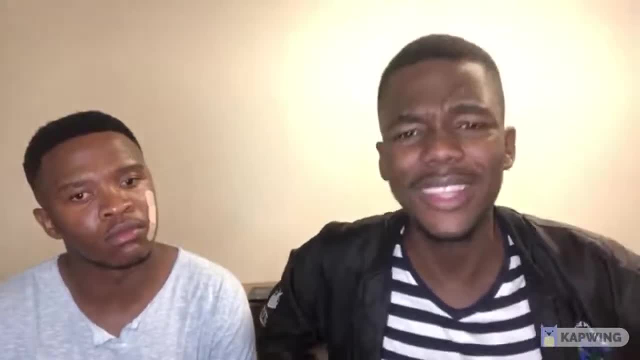 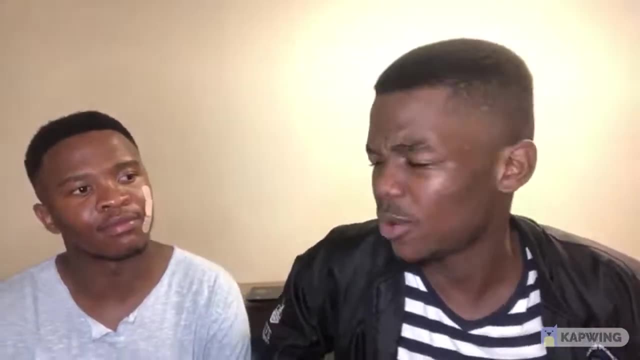 You see someone is watching, they say: okay, we can hear that you are dealing with maths and all that stuff. So, like in terms of employment, I can work as a watch. Okay, since what I said, it's mathematical statistics and also financial orientation. 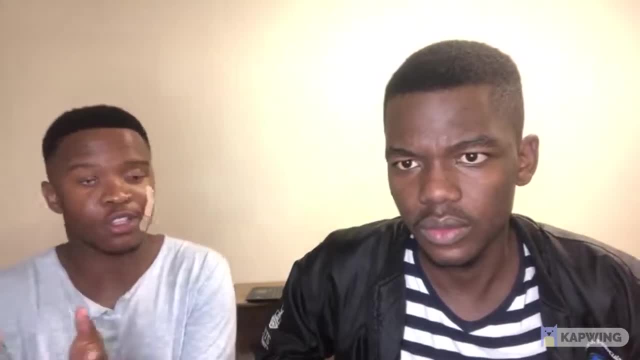 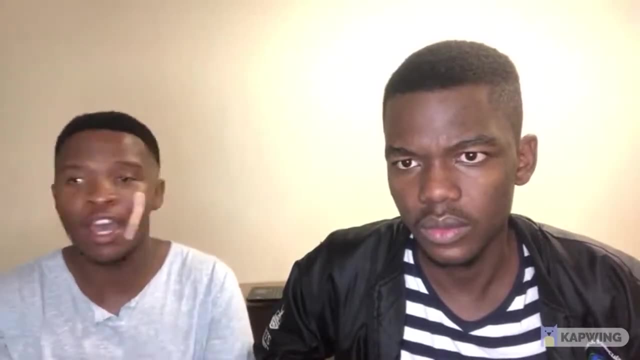 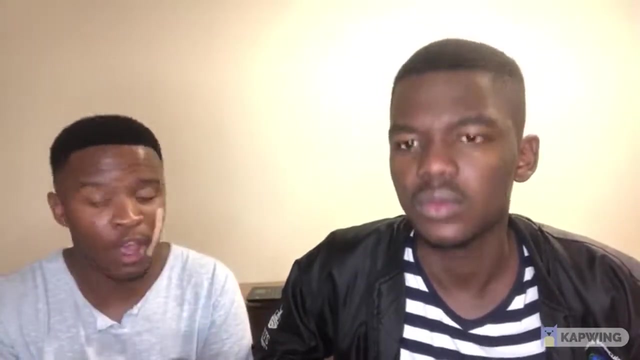 Remember finance. it has its own careers like risk management, all that, and then statistics. it also has data analysts, researchers and all that because as a statistician, you have to collect the data from everywhere, then you have to analyse it, then, after analysing, 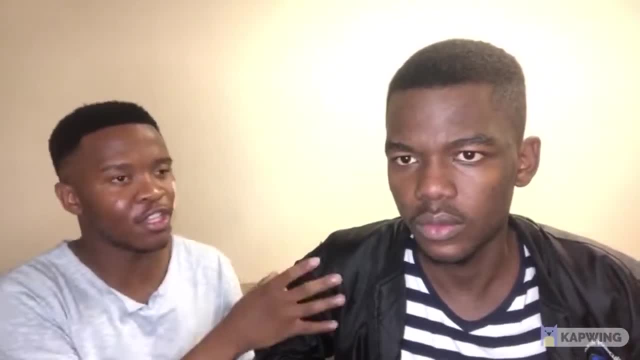 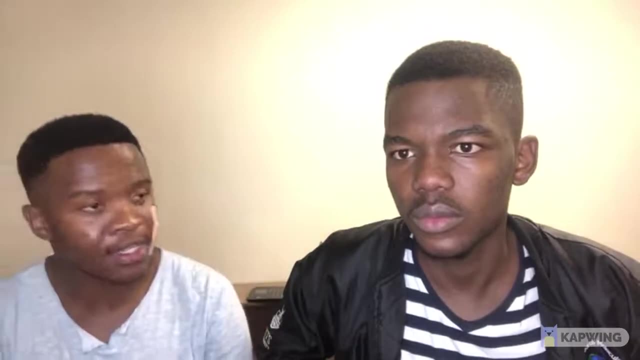 it. you have to summarise it because if you are the CEO of the company, you don't know many things, then as a statistician, I have to collect that data, analyse it and, after analysing it, I have to summarise it. then when I have to display it to you, you have to understand. 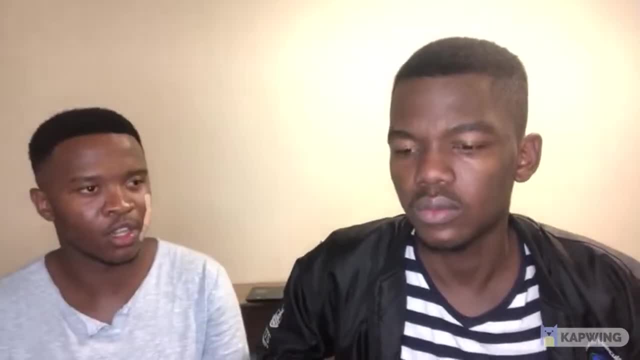 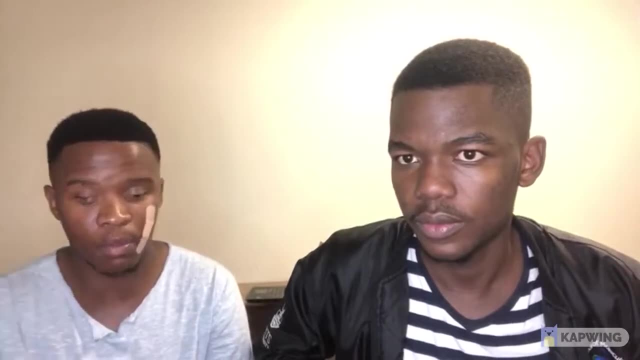 what's happening like I have to give you something that you can read. you get it. Yes, Same as accountants most of the time. yes, yes, And some of them, with this degree, they become teachers. yeah, some of them, they want to. 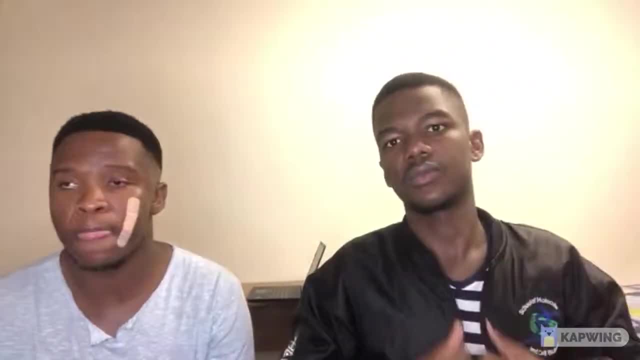 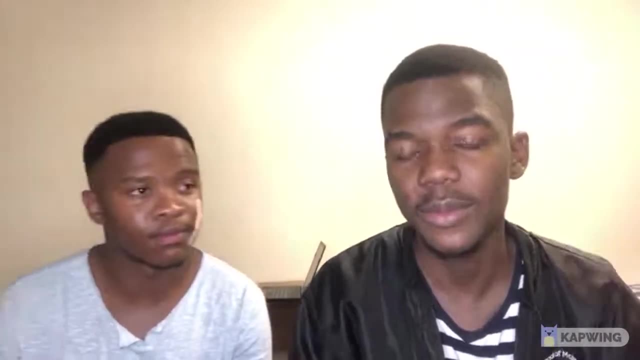 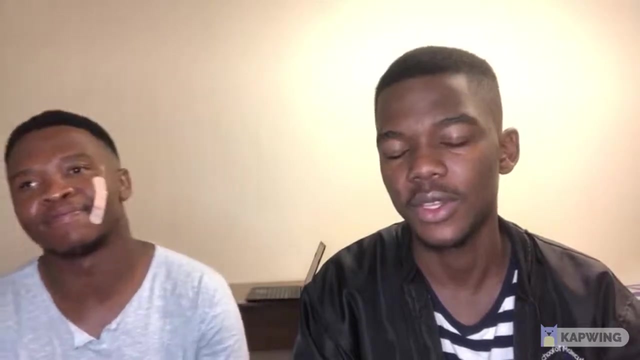 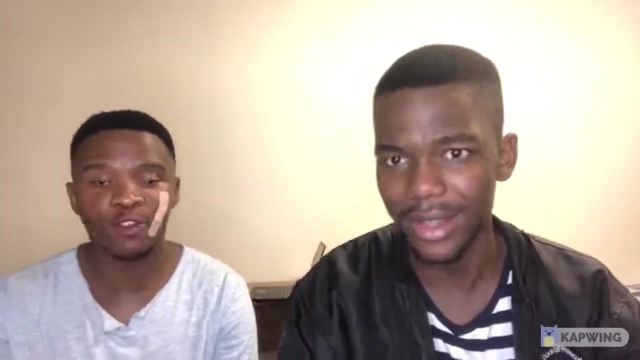 be lecturers, and it is possible. it is possible. yes, There's a majority of opportunities. yeah, it's mathematical statistics. yeah, wow, great, you can become a statistical analyst, maybe also a statistician. yeah, yeah, yeah. 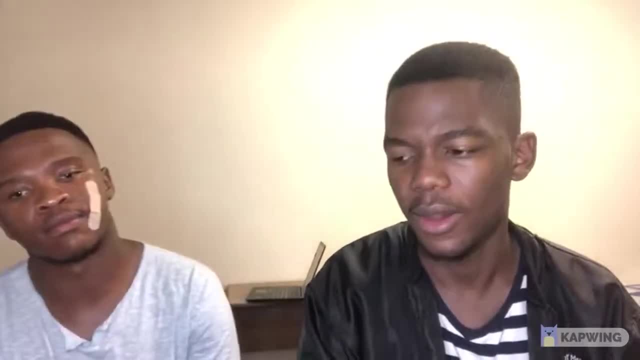 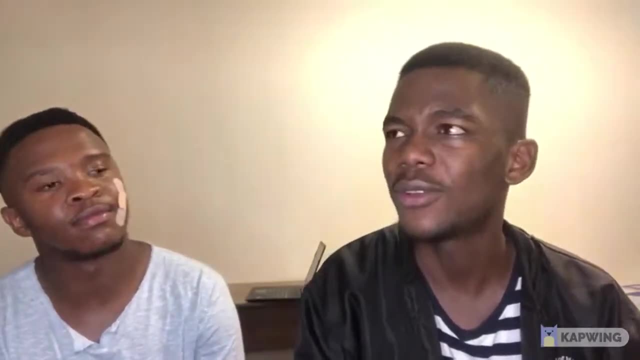 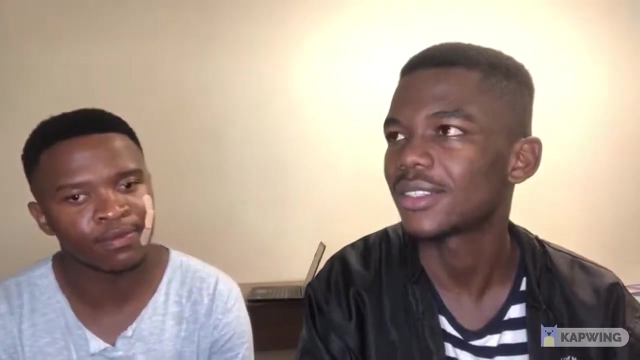 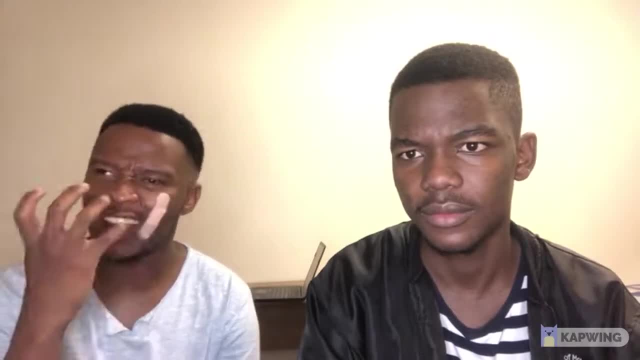 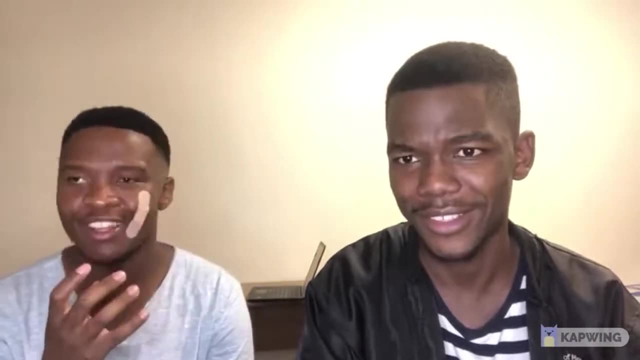 now is that you have to have in-guard. I don't know if you guys understand this in-guard like you have to have that thing. I've already. you have to be stubborn. you have to be stubborn with this thing because, um, it's tough, it's never. 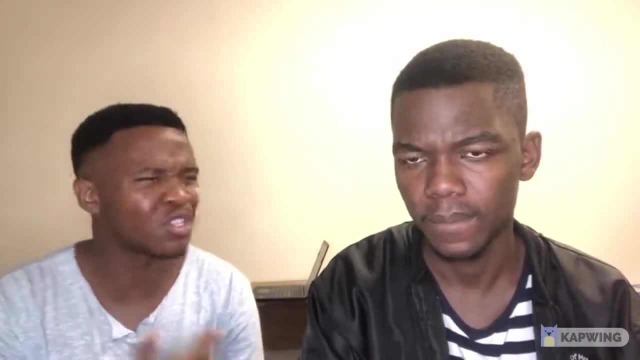 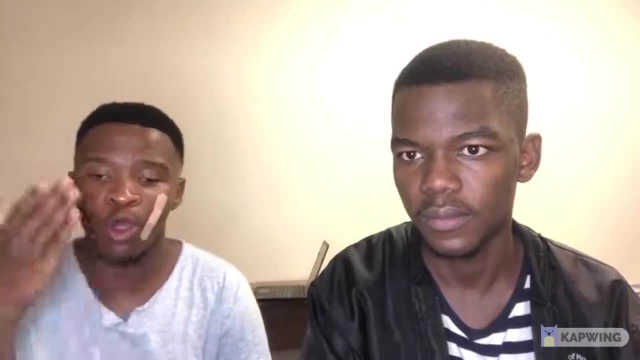 easy, you get it, but if i'ma tell you that, ah, the course is chowing because as friends we are not the same. you can text me: what are you doing? i'm just um going out, uh, what, what, what, what. but you and i, we all know that we are here for a reason. you understand. many people come here, then they. 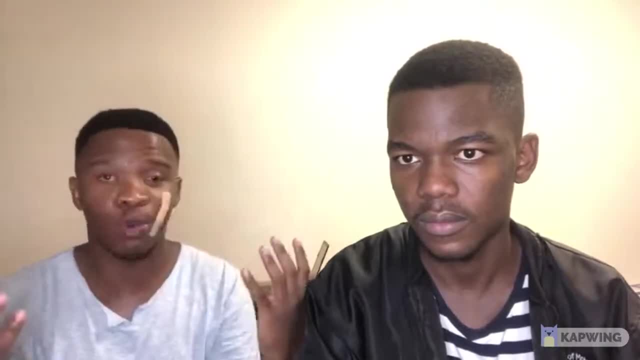 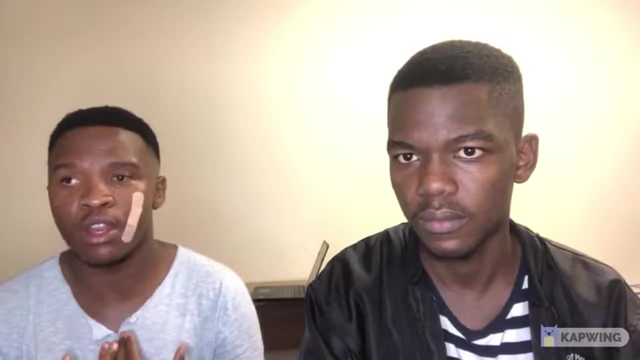 cannot be introduced to all these um, nice things around job, then they kind of forget where they are from. you understand, when they fail, then they have to go, go back, because some of us, we, we remember that, uh, when we're coming back, we have to fix the situations. you get it. so we are here. 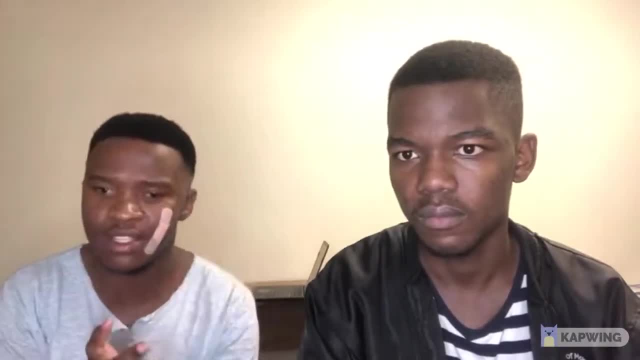 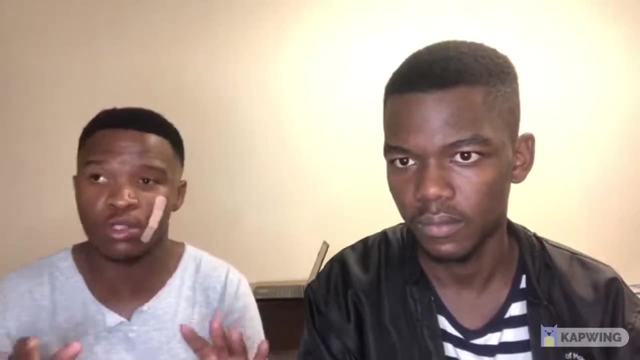 for a reason. so the only thing: if math is tough, statistics is tough. statistics is not nice. but if you work hard with our friends and all that, you can even set up a meeting with a lecturer. they are so nice, you know, guys are paying them, so they have to do their work and you get it then uh, 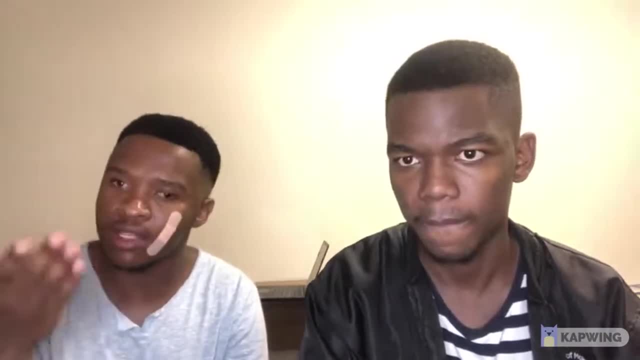 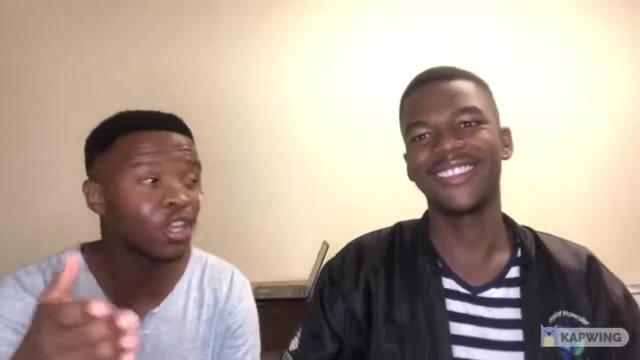 what i can say is to um, you have to work hard. if you don't understand us, then uh, this thing i worry. if you are stressed, you have to drink alcohol. that's not the solution, because you can drink in the morning. that's some that moved you yesterday. it will come back it.